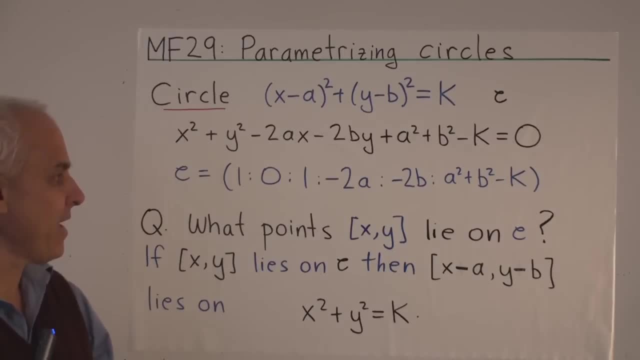 How is that term in a list? This proportion of six coefficients effectively captures what a circle is, and in fact that's how we defined officially what a circle was. The question we want to talk about today is: when does a point xy lie on such a? 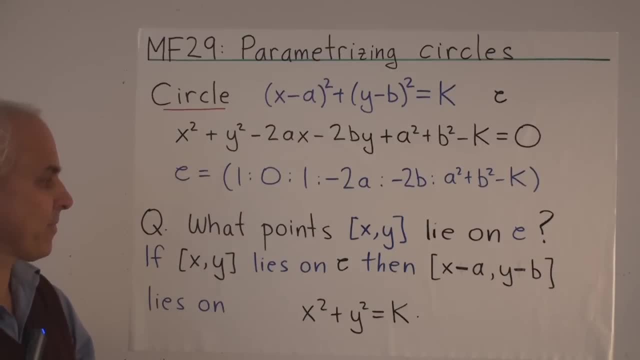 circle and which points lie on such a circle. It's made simpler by the observation that if x and y satisfy this equation, then x minus a and y minus b satisfy this somewhat simpler equation. x squared plus y squared equals k. And since going from xy to x minus a, y minus b is simply as a shift, we can without. 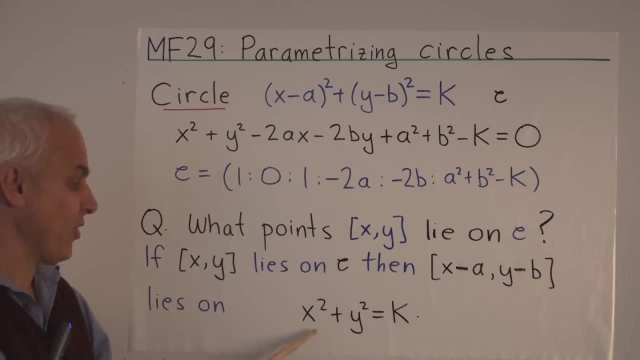 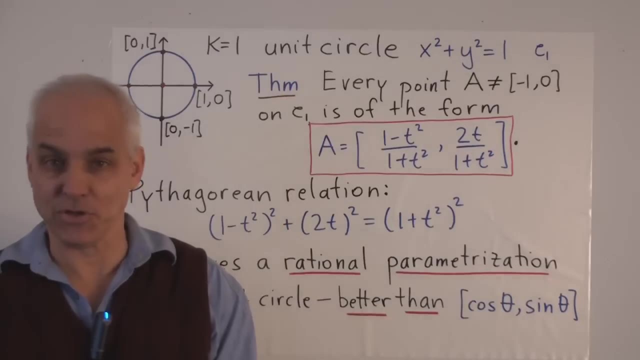 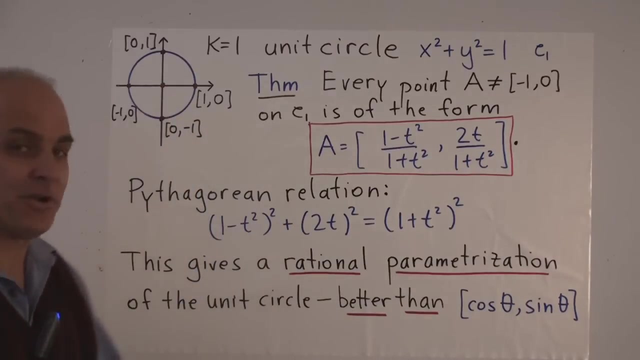 loss of generality, restrict ourselves to simpler circles of this kind, circles whose center is at the origin. So let's have a look at the simplest possible circle, the unit circle, with equation: x squared plus y squared equals 1.. There it is, there with center 0, 0, and it goes through the points 1,, 0,, 0,, 1,. 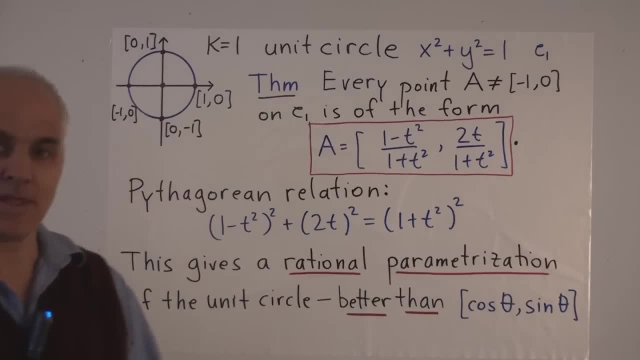 minus 1, 0 and 0, minus 1.. But it actually goes through a lot of other points as well. How do we get those other points? Well, you may remember that 3,, 4,, 5 triangle is a right triangle, So 3, this one. 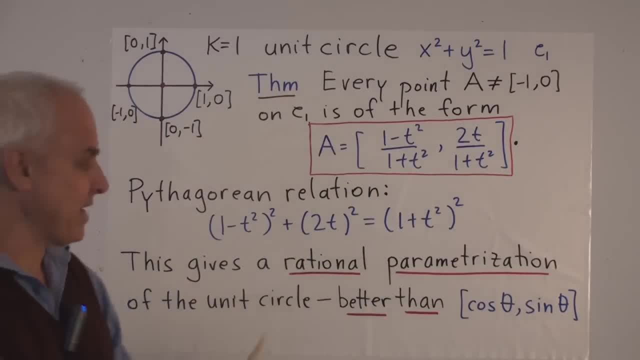 4. this way, 5 hypotenuse, that's a right triangle. That's telling us that 3 squared plus 4 squared equals 5 squared. And if you divide by 5 squared you get that 3 over 5, all squared, plus 4 over 5, all squared equals 1.. So the point 3: 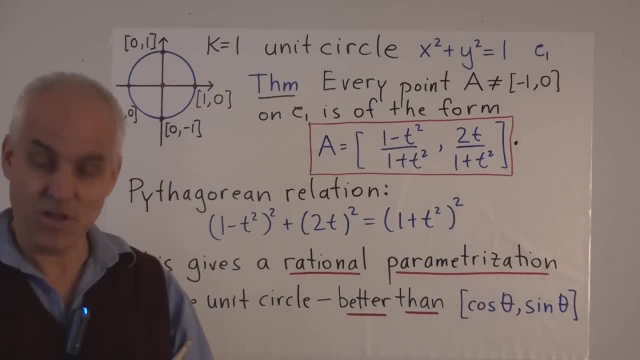 fifths. 4 fifths is also a point on the unit circle and it comes from Pythagorean triple And that's a general kind of phenomena which is captured by this theorem. Every point on this circle, with the exception of minus 1, 0, can be written in: 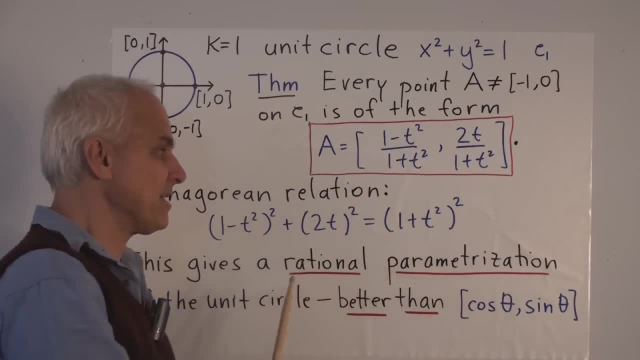 this following form: 1 minus t squared over 1 plus t squared. 2t over 1 plus t squared When t is 0, we're here. when t is 1, we are here. when t is minus 1, we are. 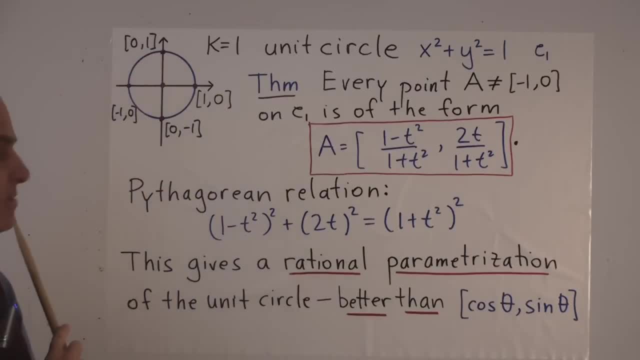 here and as t gets bigger and bigger, we approach this point. When t becomes a bigger and bigger negative number, we approach this point from the opposite direction. Naturally connected with this parameterization is this identity or this relation That if you take 1 minus t, squared and square it, and take two t and 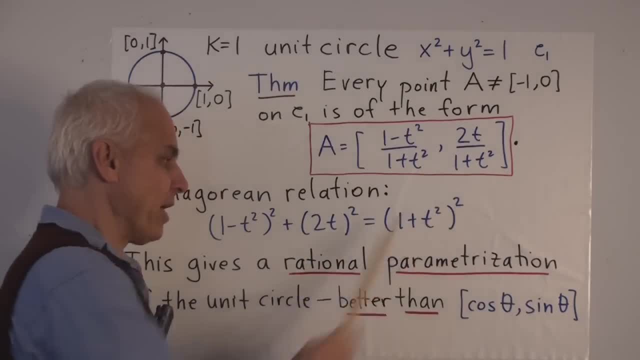 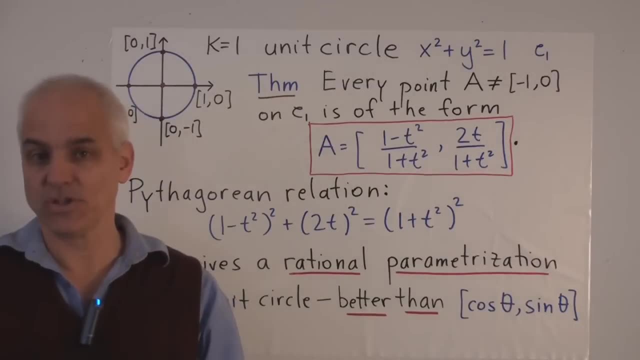 square it and you add them, then you get exactly 1 plus t, squared, all squared. This rational parameterization of a circle, of the unit circle, is very useful and important and, for many applications involving circle geometry, its preferable to the more usual familiar parametrization. 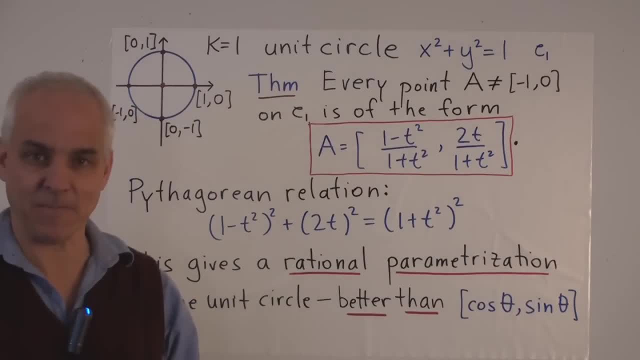 involving the transcendental circular functions cosine and sine. The problem with this parametrization is that it's almost never accurate. If you actually want an example of a number of a point like this, you plug into your calculator. it spews out some answers to ten decimal places or whatever. 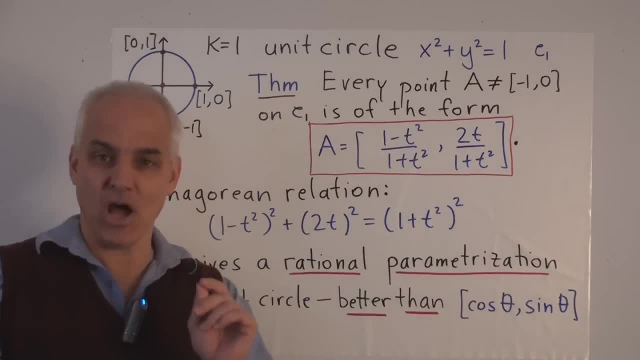 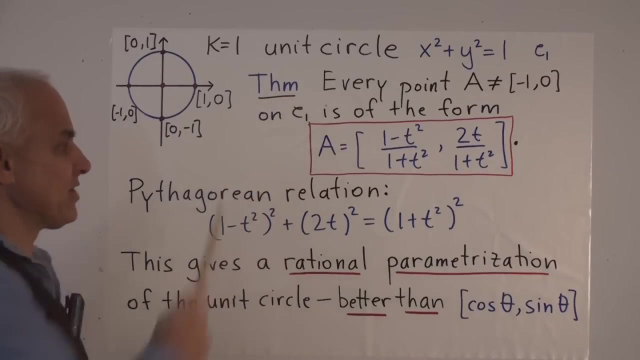 and you get a point which is approximately on the circle, but not exactly on the circle. This parametrization- we're still dealing in 100% accuracy, which is what we want, because we want to do mathematics completely correctly. Now let's see how this result. 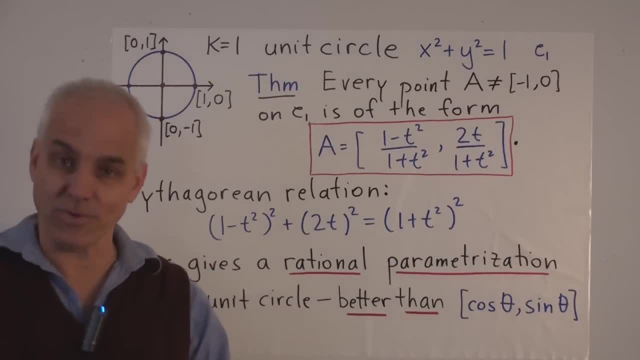 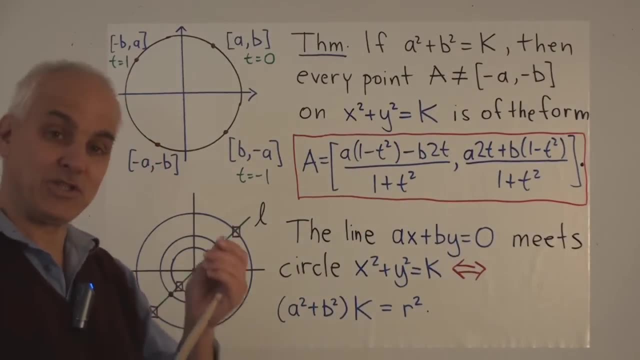 this parametrization of the unit circle extends to a more general circle. Now let's have a look at the general circle. with equation: x squared plus y squared equals k, We'll assume that there's at least one point on the circle. say a, b. 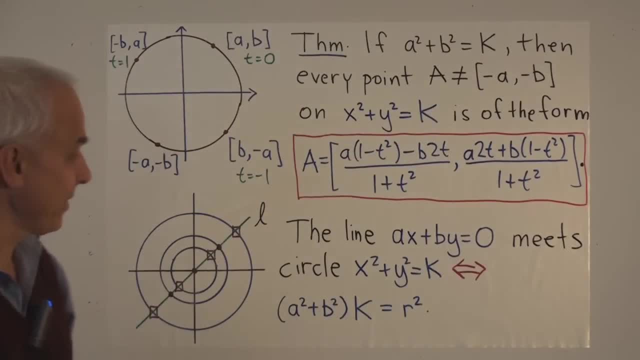 so that a squared plus b squared equals k. Then there's at least these other points, minus a minus b, minus b a and b minus a, which are also on that circle. How do we parametrize the points on this circle? 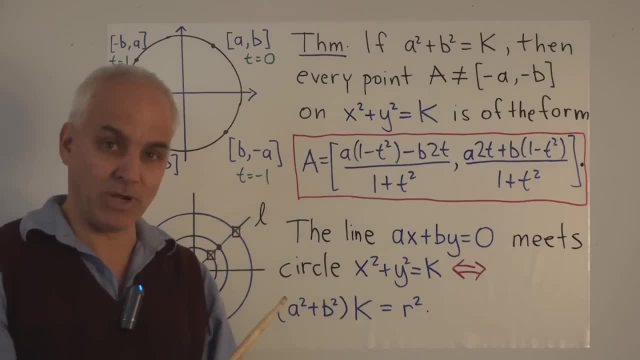 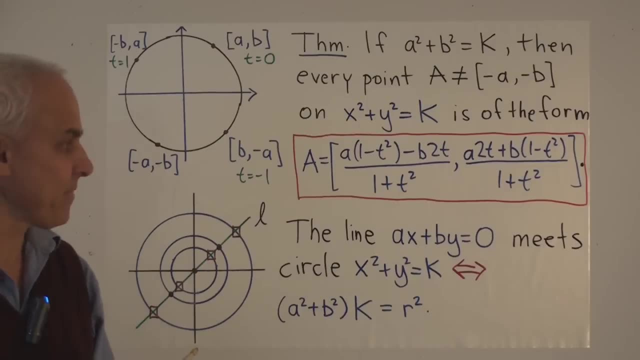 Well, it's a little bit different, a little bit more complicated, but it's the same generalized idea. as for the unit circle, Every point on this circle, with the exception of this minus a, minus b, can be written uniquely in this form. 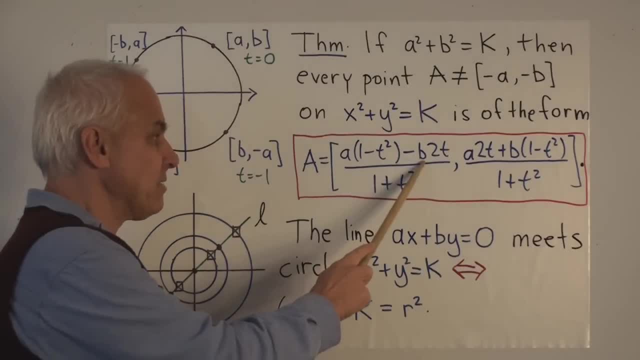 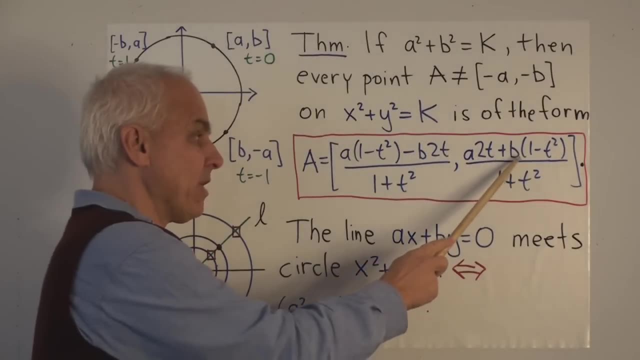 Next question: What is the coordinate a times 1 minus t squared, minus b. times 2t, all over 1 plus t squared, And y coordinate: a times 2t plus b. times 1 minus t squared, all over 1 plus t squared. 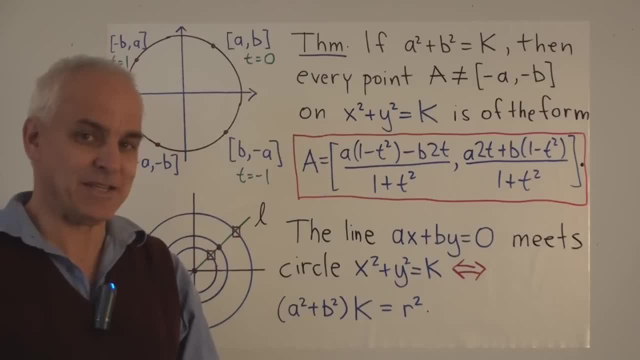 So that's a theorem that follows in a similar way as does the previous one. It gives a complete parametrization of a general circle. One of the interesting features about geometry with circles is that a line is a line and a line is a line. 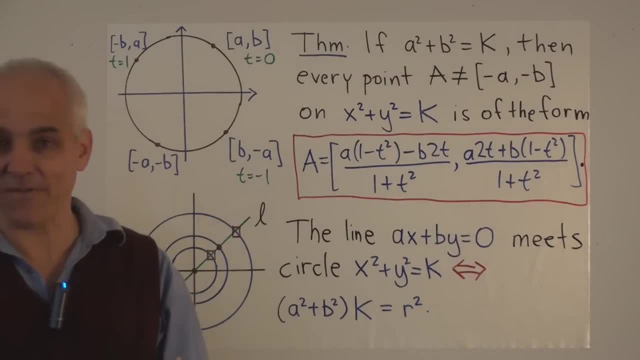 and a line is a line, and a line, through the origin or the center, does not necessarily have to meet the circle. Whether it does so or not depends on number, theoretical considerations. And so we get a link between geometry, very simple geometry. 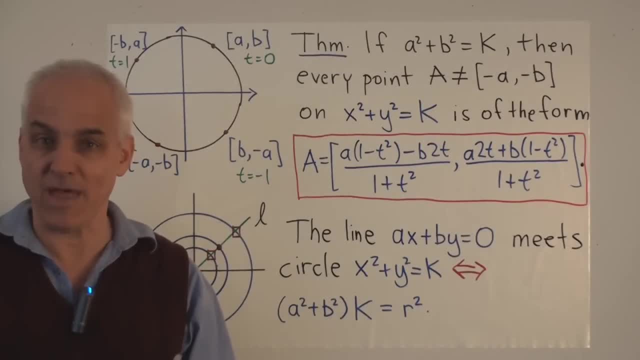 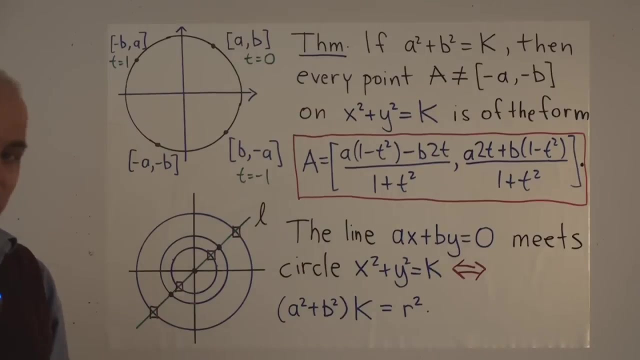 and classical problems in number theory that have been around for thousands of years, that were studied by Euclid, that were studied by Fermat and his contemporaries. So the situation in general here, with the circle of the form, x squared plus y squared equals k. 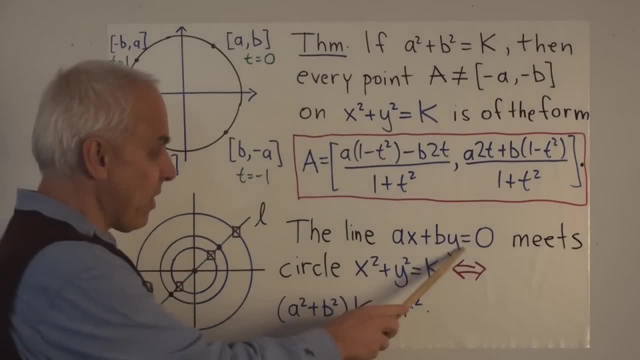 and a line through the origin of the form ax plus by equals 0, is that the line meets the circle precisely when this number theoretic condition is satisfied. When a squared plus b squared times, k is a square. When we say it's a square, 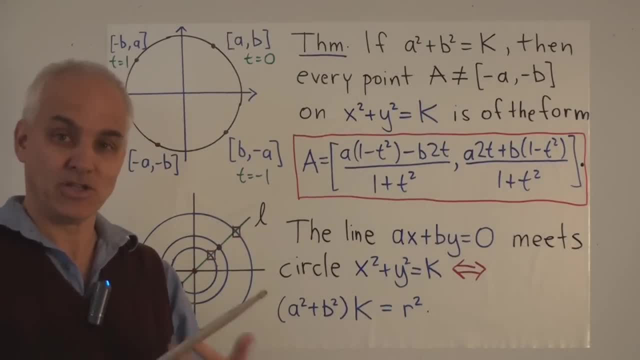 we mean that it's a number, a rational number- r squared, And so this line, this line l, may or may not meet a circle through the center there. So this is a little bit of a different aspect of circles than you're used to when you deal with real numbers. 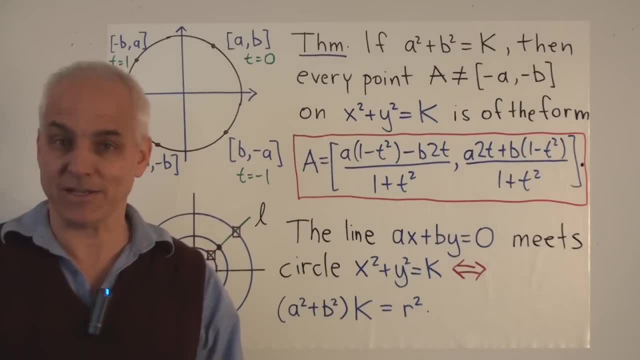 With real numbers, a lot of arithmetical subtlety vanishes from geometry. So one of our aims is to bring back this natural number theoretical aspect of geometry into elementary geometry also. So in our next video we're going to have a look at another important concept. 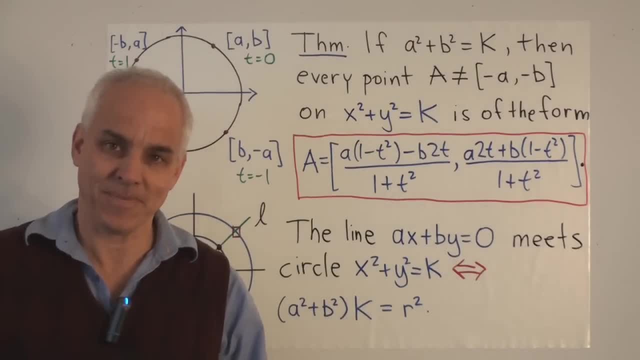 from elementary geometry, the idea of a vector. I hope you're going to join me for that. I'm Norman Wahlberger, and thanks for listening.